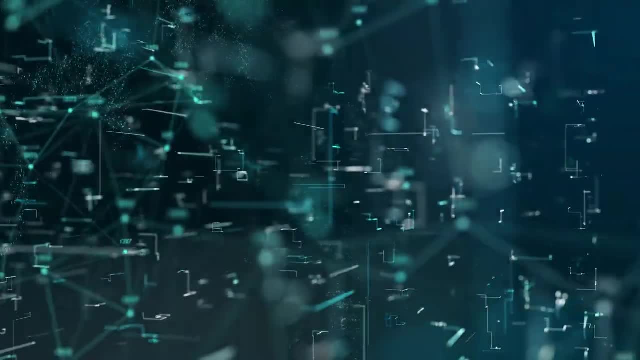 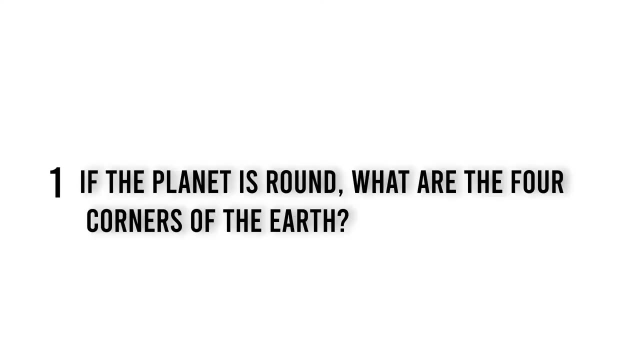 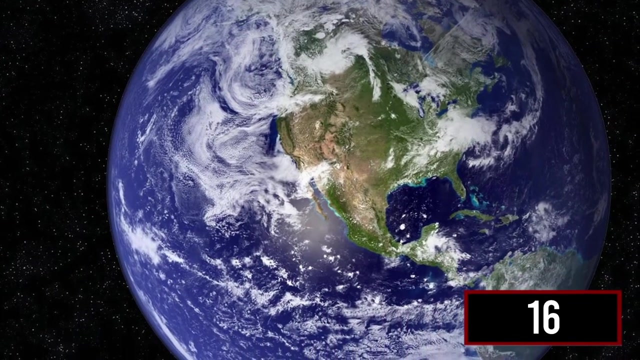 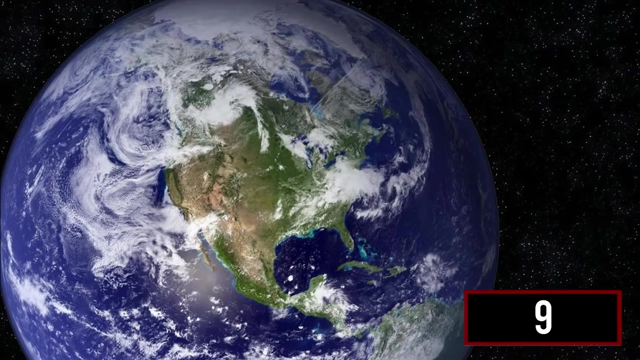 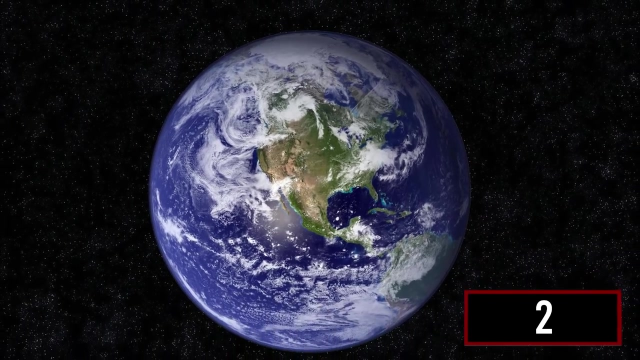 Stay until the end, because the last question is the most important. Let's get to the questions. Question 1. If the planet is round, what are the four corners of the earth? The four corners of the earth are believed to be a metaphor for talking about the four 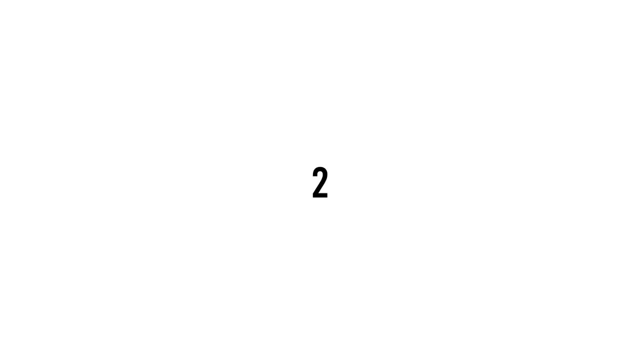 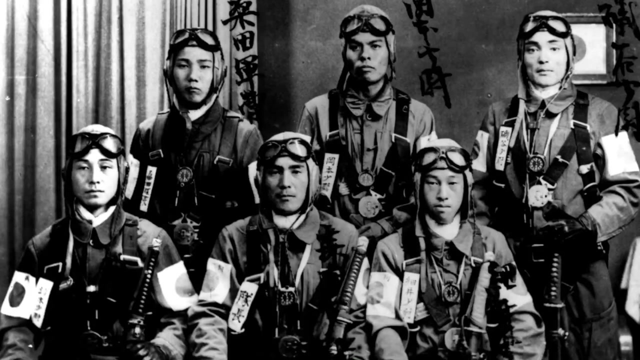 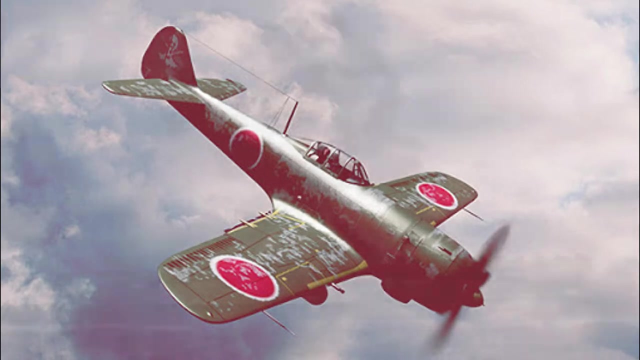 cardinal points: north, south, east and west. Question 2. Why did the kamikazes wear a helmet? But what are the kamikazes? In World War II? there were Japanese suicide pilots who carried explosives in their planes and threw themselves on enemy ships, so they sacrificed themselves. 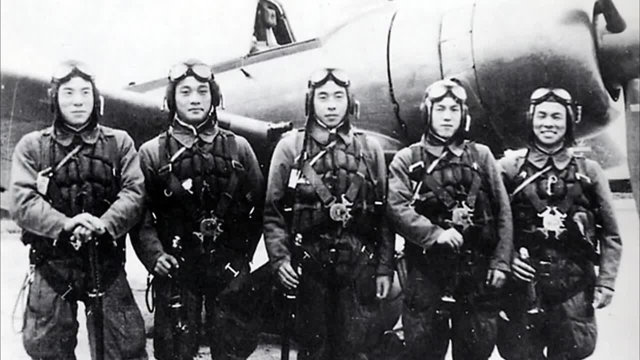 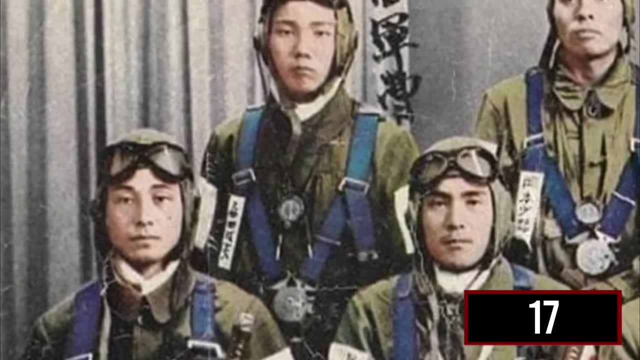 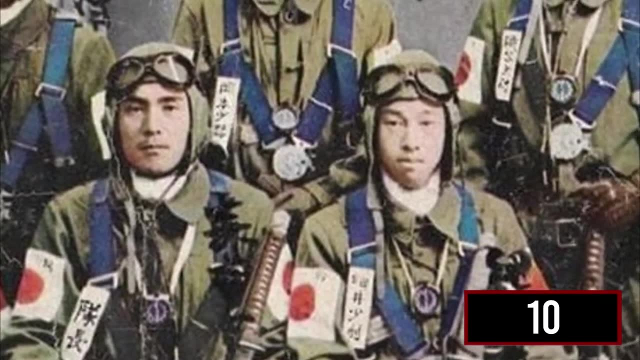 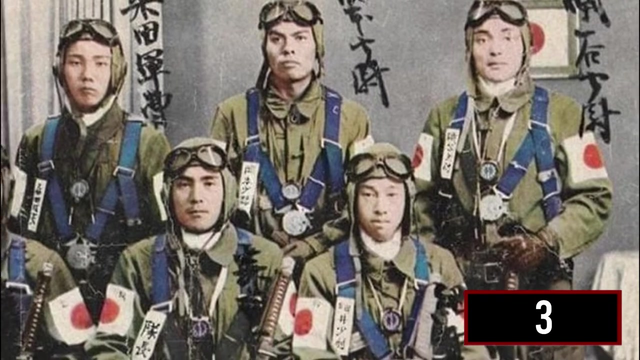 to defend their country. these pilots were called kamikaze. So the question arises: why did they wear helmets? There is a Japanese helicopter that has this helmet attached to its sixteen noses. However, there was a Sri Lankan uncertain about whether this helmet would worn out or not. 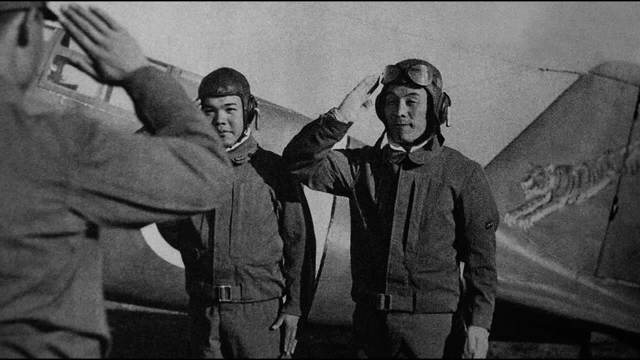 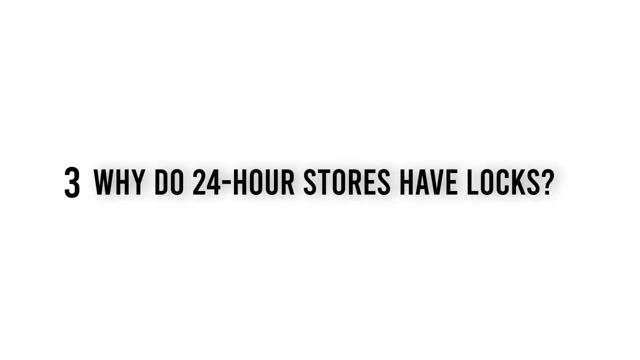 when the kamikazes took off. The Kamikazes wore helmets because if the mission failed, the helmets would increase the pilots chances of surviving. Question 3. Why do $$$, $$, $23.. INCREASE, INCREASE IN CONSENSUS OF ENERGY? 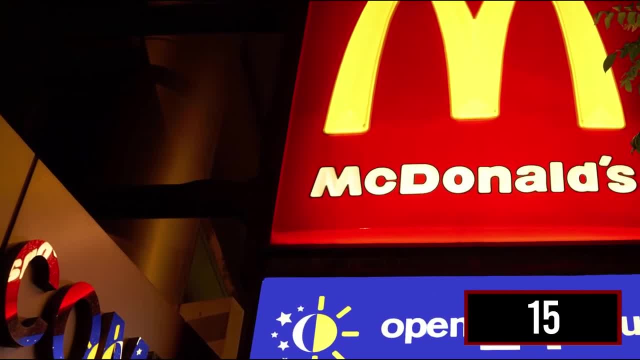 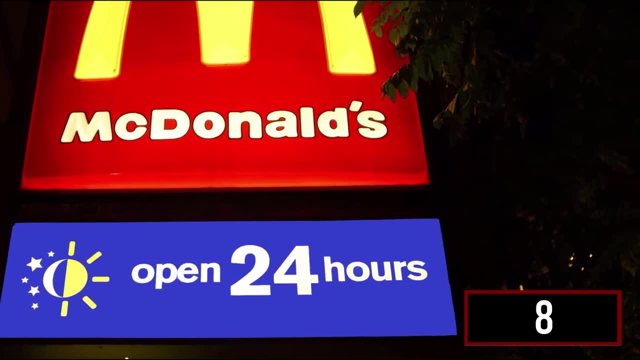 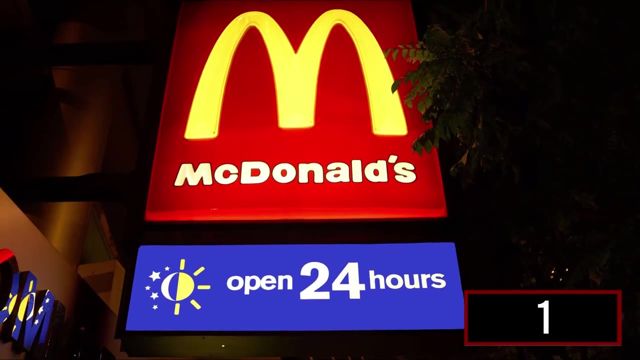 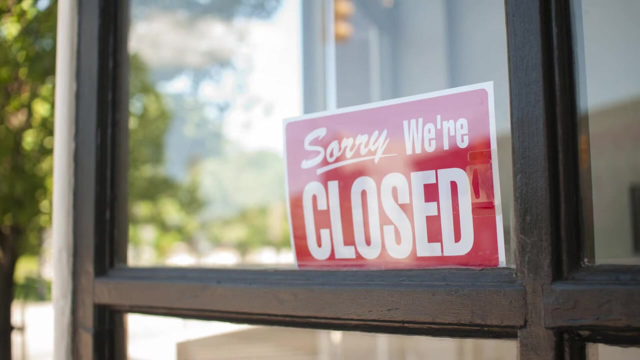 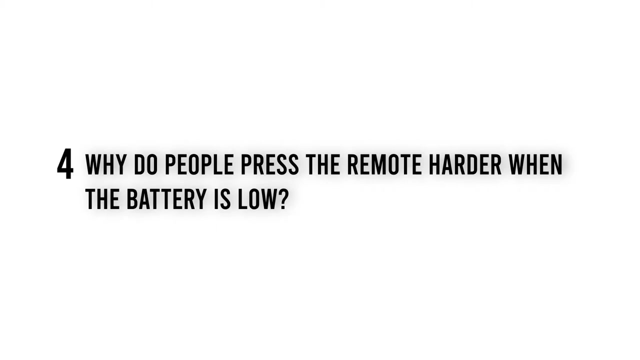 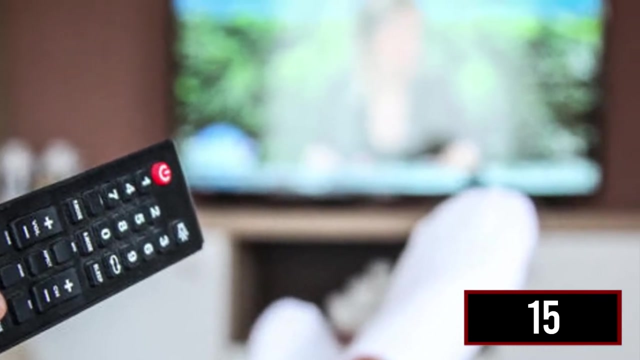 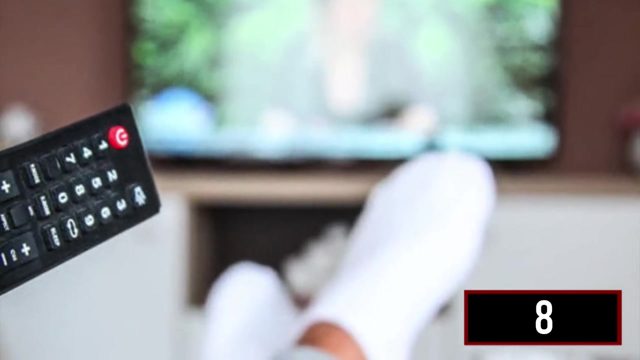 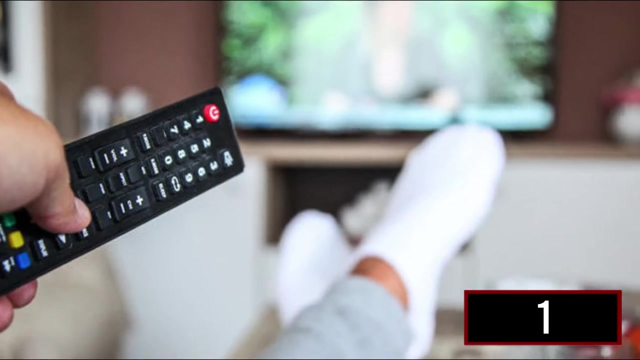 Why do $$$, $$, $3. INCREASE IN CONSENSUS OF ENERGY? 24-hour stores have locks because they may need to close at some point, for example, a holiday, renovation or cleaning. Question 4.. Why do people press the remote harder when the battery is low? 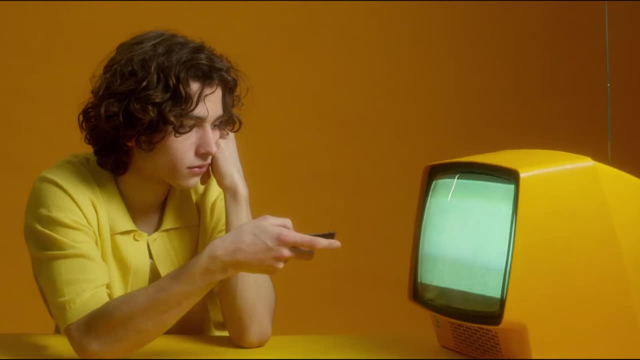 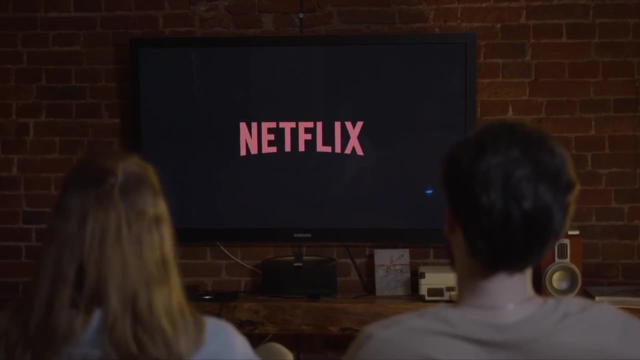 When we take an action and the result is not what we expected, one of the effects is to increase the magnitude and frequency of the behavior. In the case of changing the TV channel if the battery is low, the instinctive tendency is to press the button harder instead of changing it. 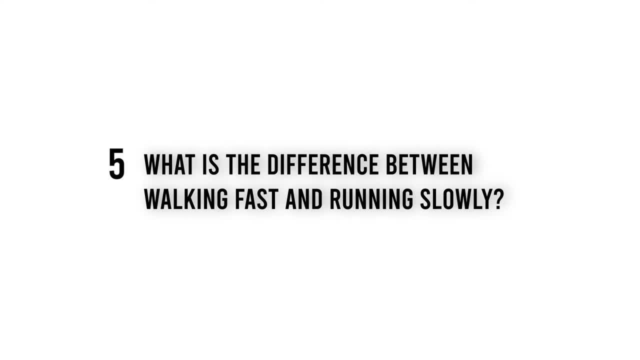 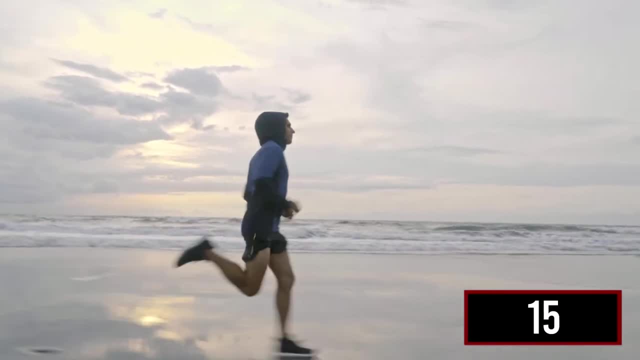 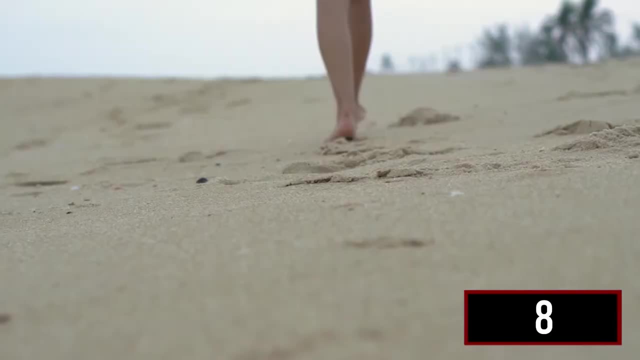 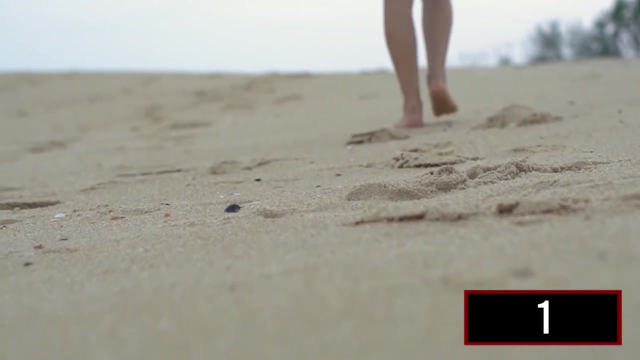 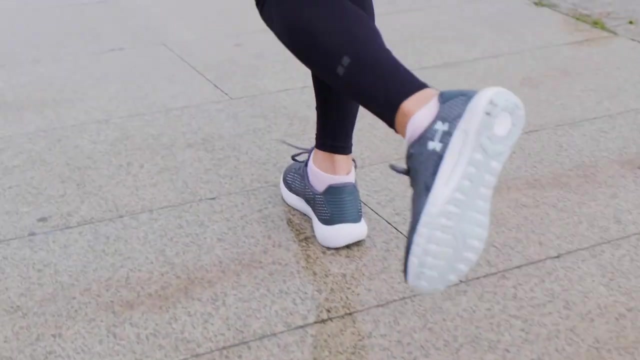 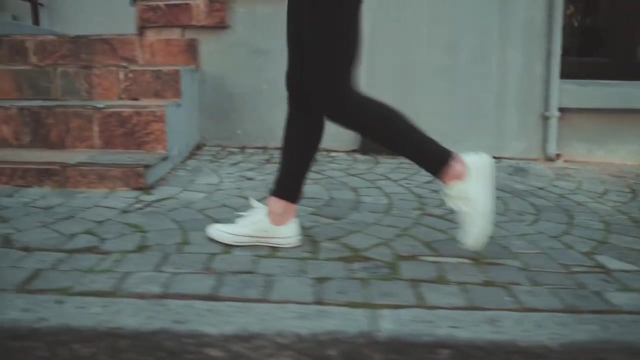 Question 5.. What is the difference between walking fast and running slowly? The difference is that in running slowly, for at least one moment of the transition of the feet, the person will be floating without any contact with the ground. Walking fast means the opposite. the person always has at least one foot on the ground. 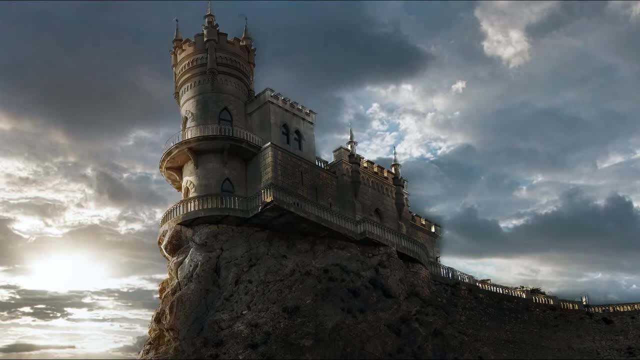 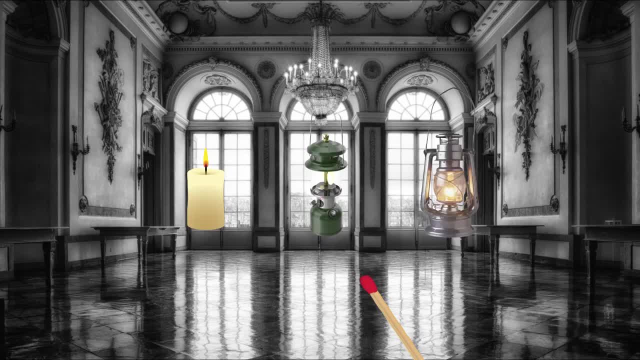 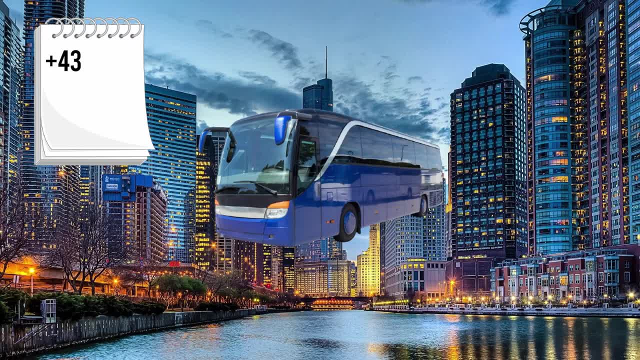 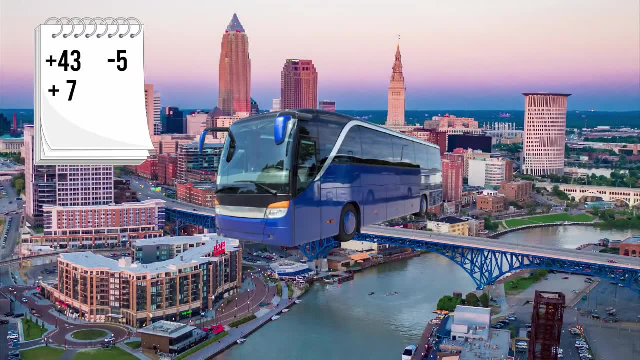 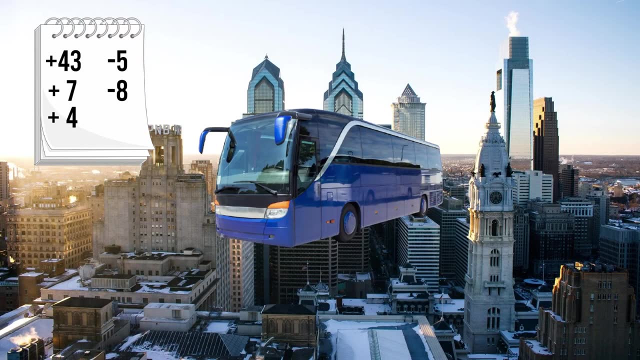 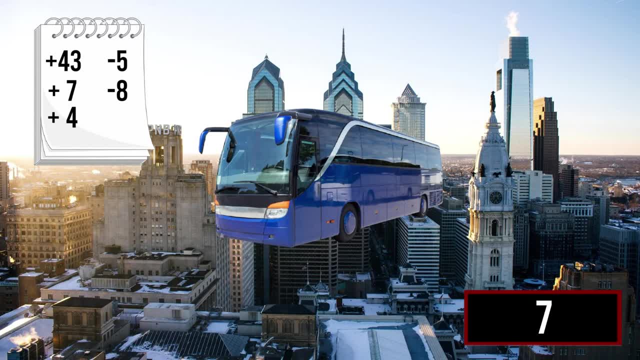 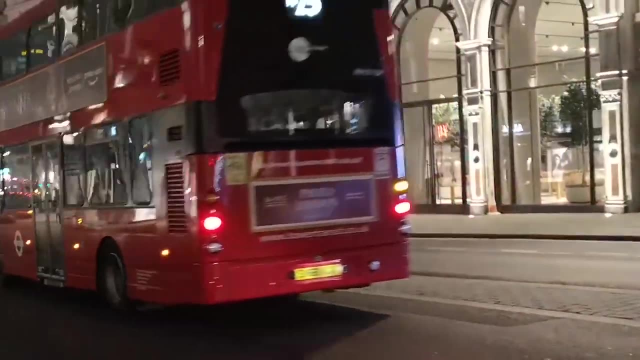 matchbox that contains only a two. You enter a dark castle with a matchbox that contains only a two. You enter a dark castle with a matchbox that contains only a two. The driver's name is your name. At the beginning of the question I said you were driving the bus, so you are the driver. Before going to the results, I have something to tell you. I'm at the beginning of my channel, so, if you can like, 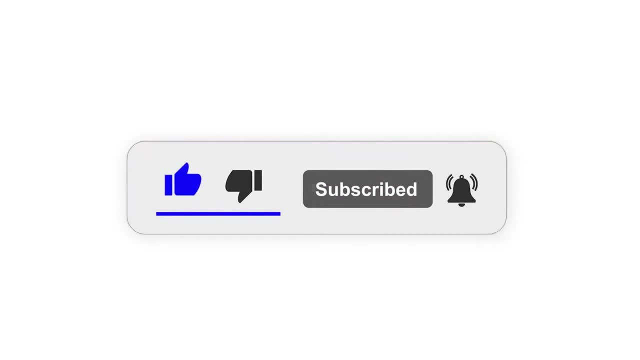 and subscribe, because in all my videos i'm trying my hardest. thank you. This test is for adults and children, so let's see your IQ. If you got it right between 0 to 2, you have an IQ of 85 to 115. 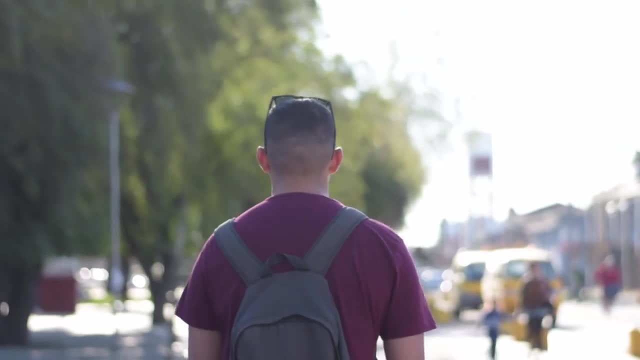 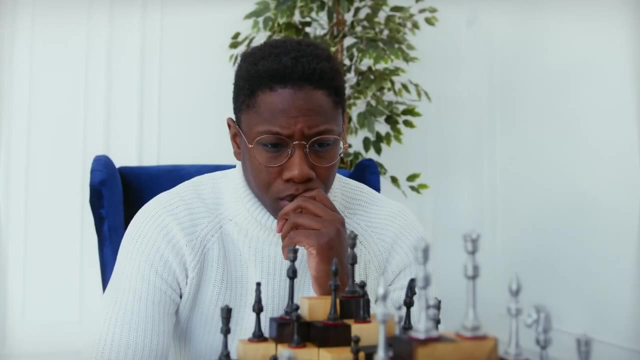 70% of the population has this IQ. I can say that you are normal. You got it right between 3 to 4. you have an IQ of 116 to 130.. 13.6% of the population has this IQ. you have above average intelligence. You got it right. between 5 to 6, you have an IQ from 131 to 145.. 2.1% of the population has this IQ. you are very supportive. You got the 7 questions right. you have an IQ above 145.. 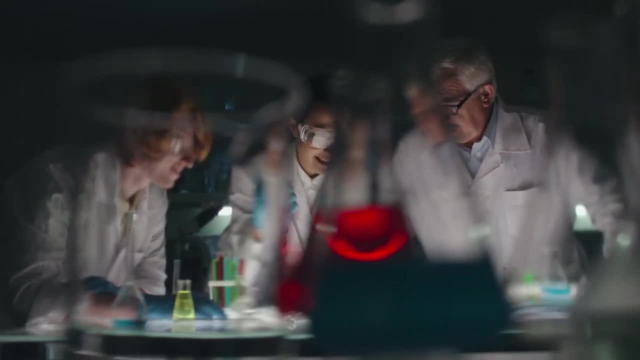 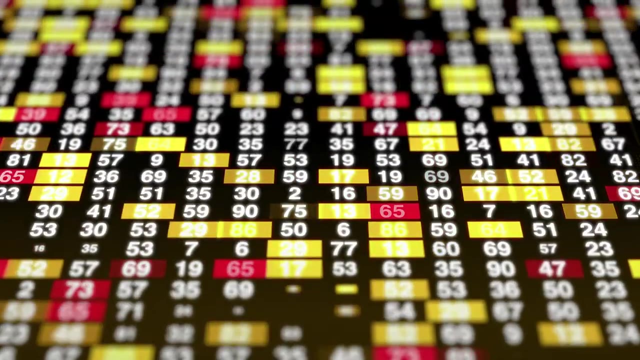 0.13% of the population has this IQ. you can consider yourself a genius. If your IQ is not very high, don't be sad. IQ is a test to train logical reasoning, but sometimes it can be a little bit difficult. 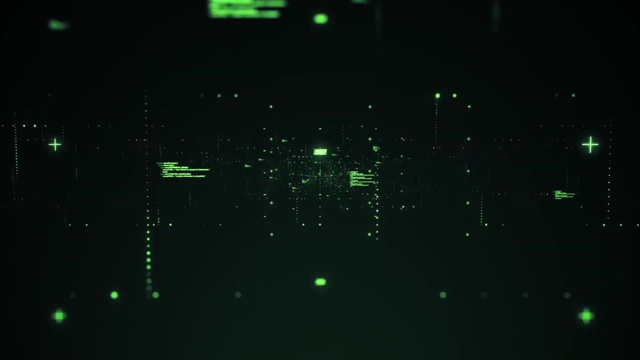 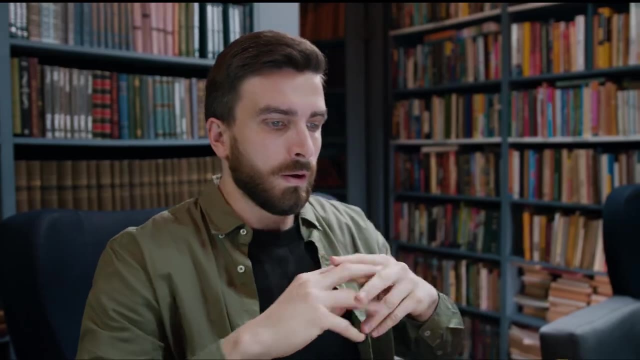 So let's see your IQ. Some people have other types of intelligence. If there was an intelligence battle between Mozart and Einstein, who would win? The answer to this fight would be difficult to answer, because Mozart has a much greater musical intelligence than Einstein, but if he had to take a mathematics test?